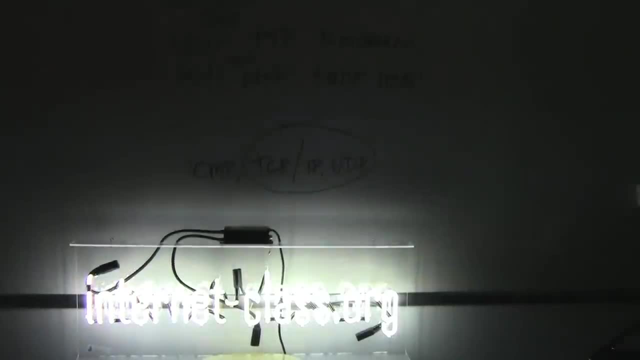 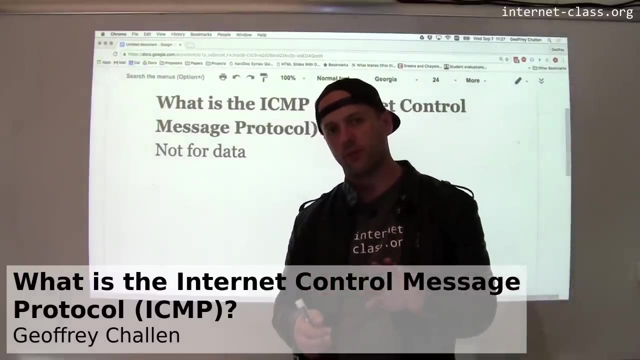 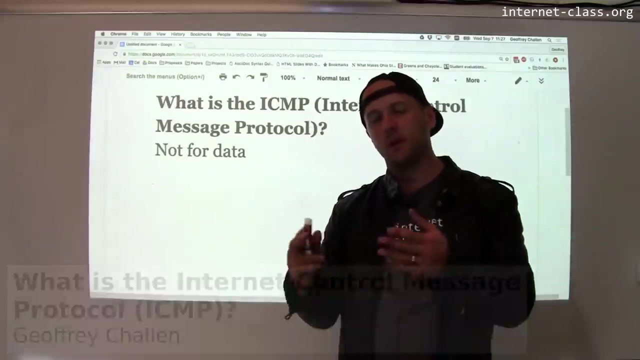 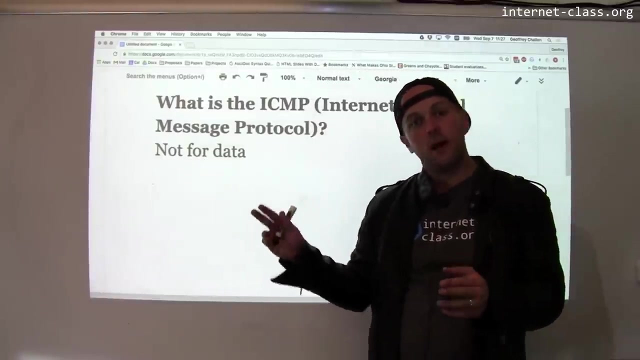 We've discussed several parts of the core internet protocol suite. We talked about the IP layer that provides best effort packet delivery between hosts. We've talked a little bit about TCP and UDP, which are used by clients to establish reliable or unreliable data transmission from one end of the internet to the other. 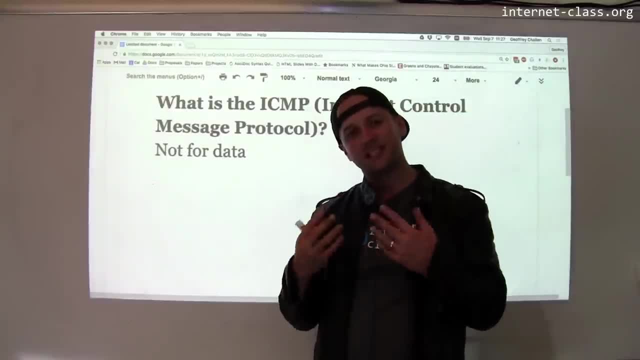 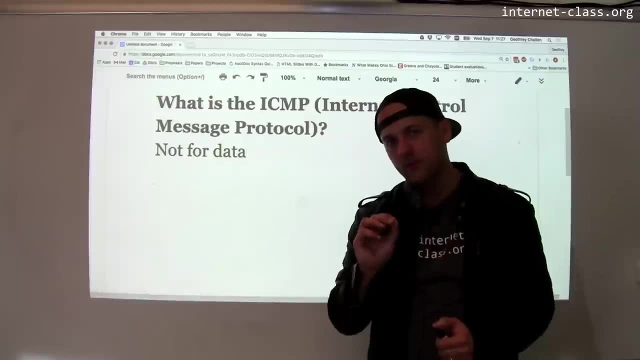 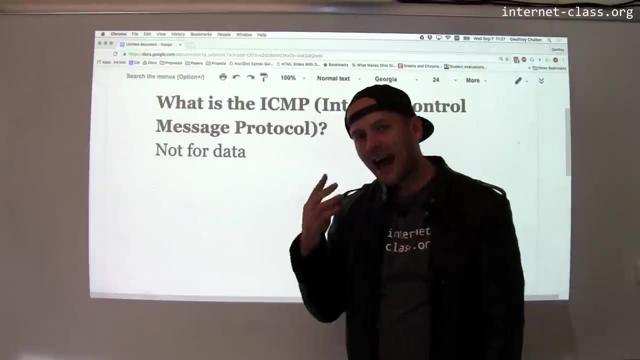 But we haven't talked about something called ICMP. ICMP is considered to be part of the internet protocol suite, along with TCP, UDP and IP, but it's actually different than those other protocols. It's referred to as the Internet Control Message Protocol and that's sort of your hint. ICMP, in contrast to those other protocols, is not for data. 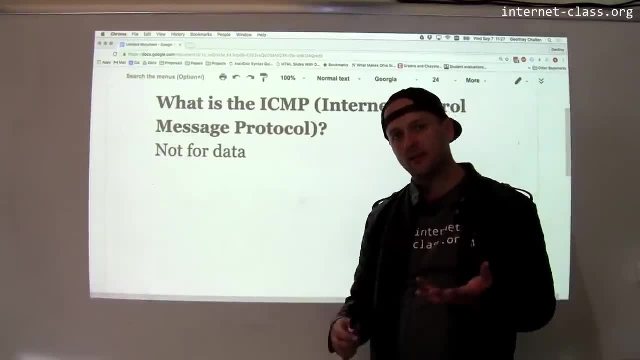 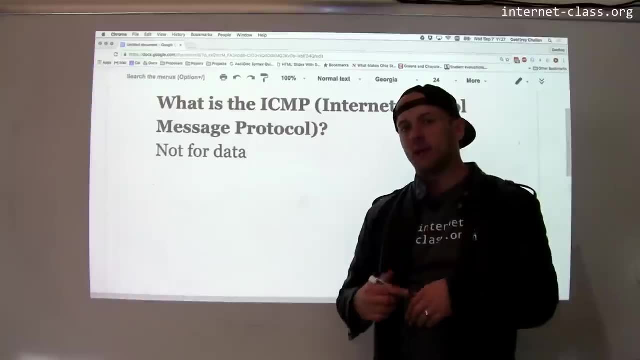 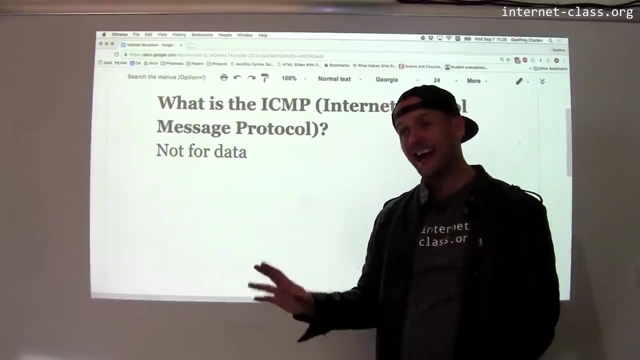 It's really designed for routers and other computers that are connected to the internet to exchange information, particularly about routing, About reachability, about- you know, did I drop a packet for a particular reason? or things like this. So this is really for exchanging information between hosts about the status of the internet and not at all for exchanging data. 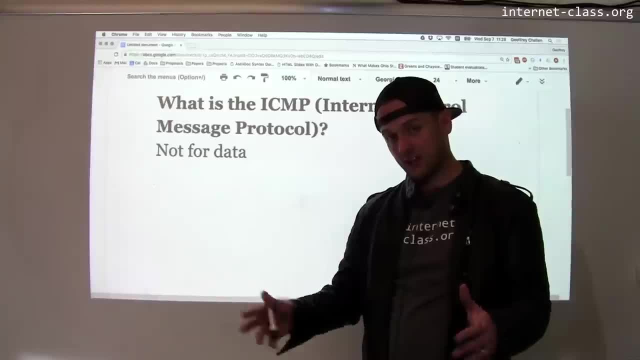 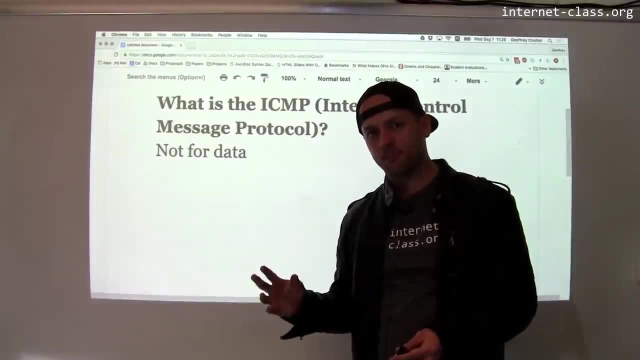 So, unlike those other tools, it doesn't move data from end to end. You can use it to sort of find out or discover interesting things about computers that are connected to the internet. A common use of ICMP, a very simple use of ICMP, is a toolkit. 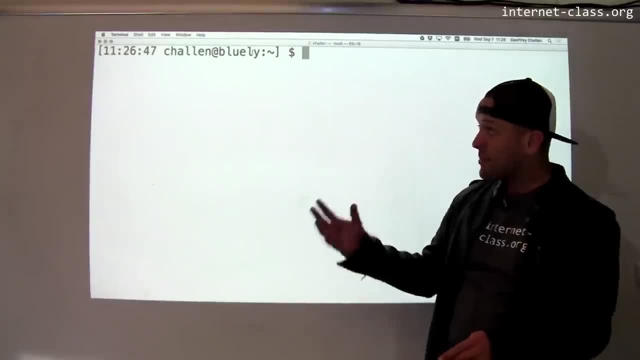 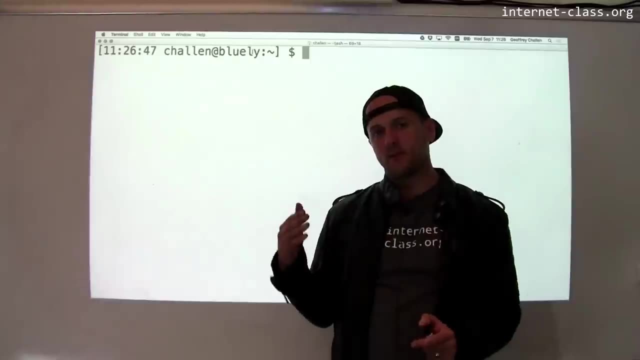 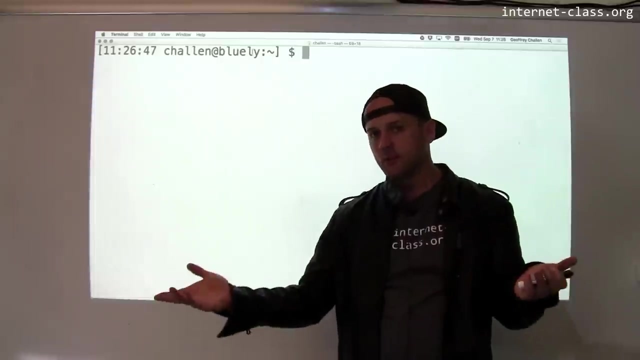 It's a tool called Ping. So you probably have Ping installed in your computer. maybe Macs sort of come with Ping. A lot of computers have Ping And what Ping does is it uses the ICMP protocol to essentially find out if a particular computer can respond to a message. 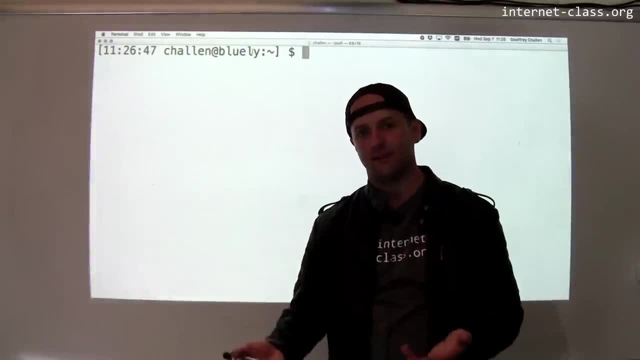 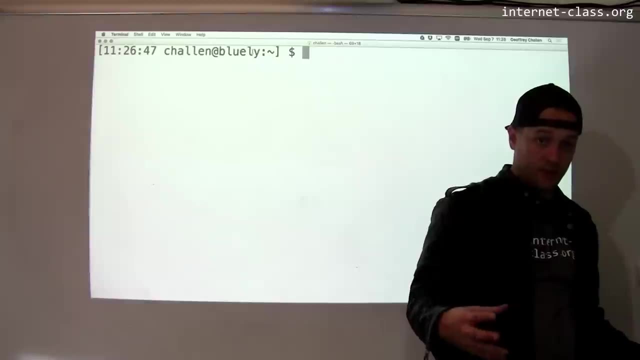 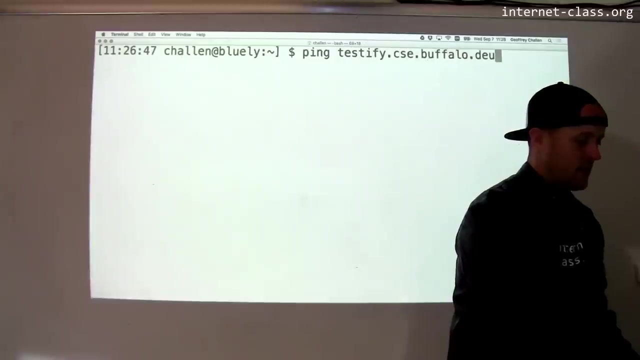 So it's frequently used for people to determine: is a computer online? So I'm here in my office. My desktop, the desktop computer that I use to do my work- is called Testify, So I'm going to run this command: ping: testifycsubuffaloedu. 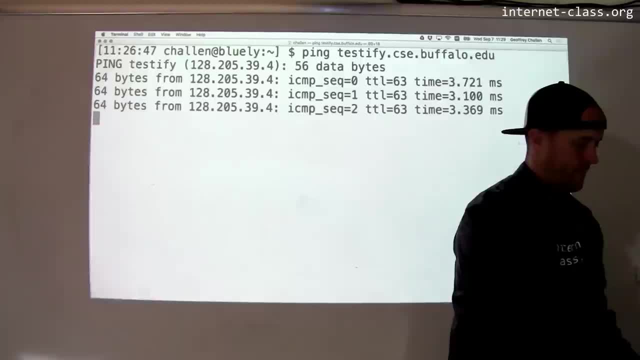 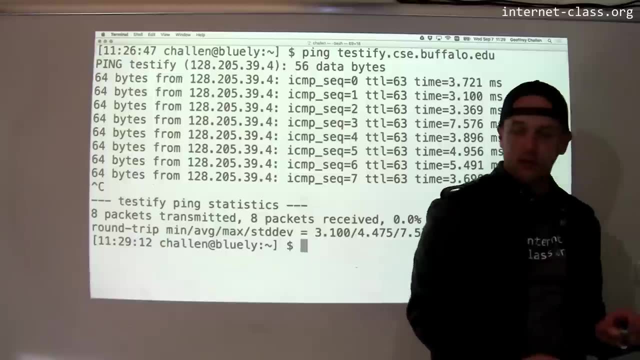 Let me just spell it right. And here's the output. And if I let this run it'll just keep going. So let me stop it and we'll look a little bit at what happened. So you can see here. this is an ICMP sequence number. 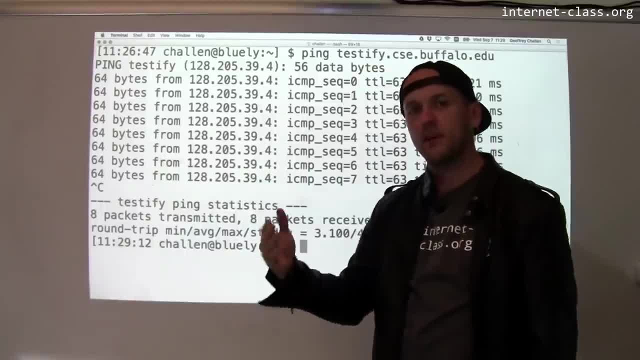 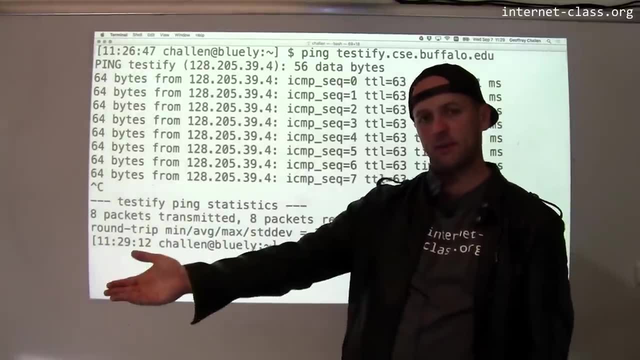 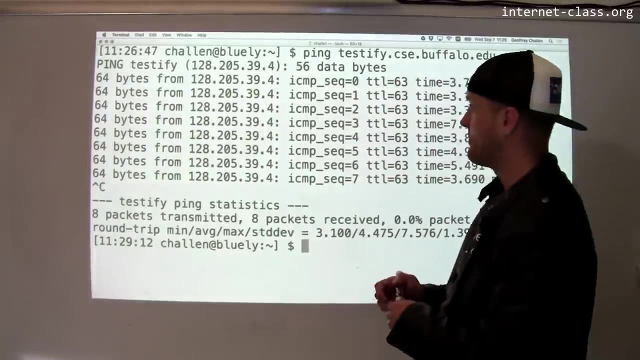 What this command is doing is it's repeatedly using ICMP to request that my computer Testify send it some information. So this is a ping. It sends a little message to Testify and Testify responds, And that's a good way to make sure that both directions of that link work. 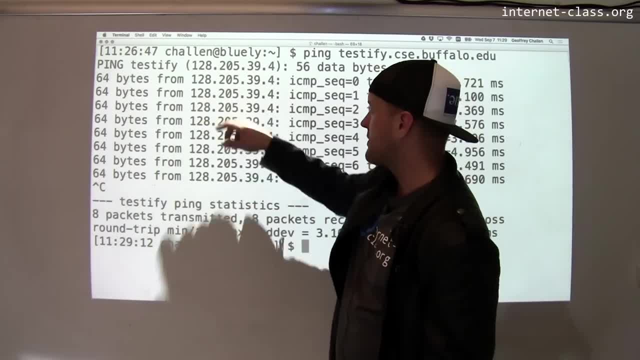 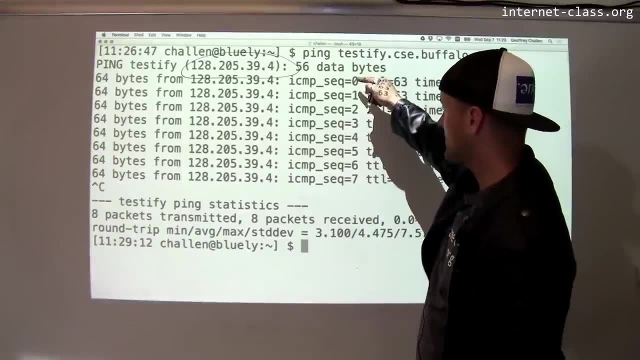 So here's an example. Let's see here. I got 64 bytes back. This is the IP address of Testify that it looked up before it ran the command. The sequence number for this ICMP goes up by one each time. This is so that I can notice if there are gaps. 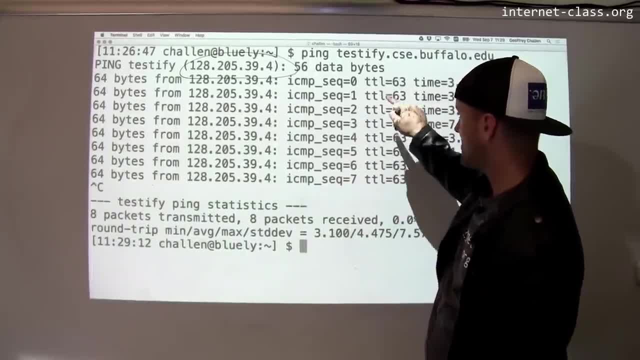 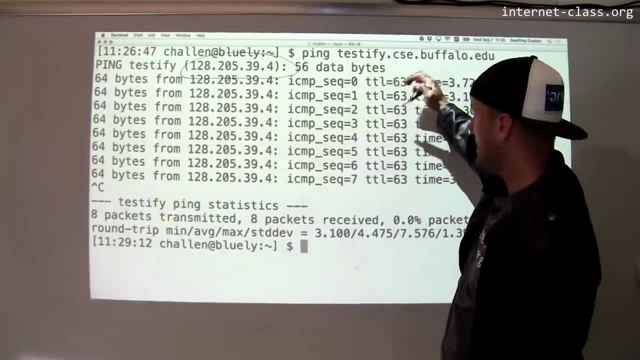 Like, for example, one of them might have been dropped somewhere. This is the time to live for the packet. So IP packets: every time they go through a particular hop, the time to live is decremented. The value probably started at 64.. 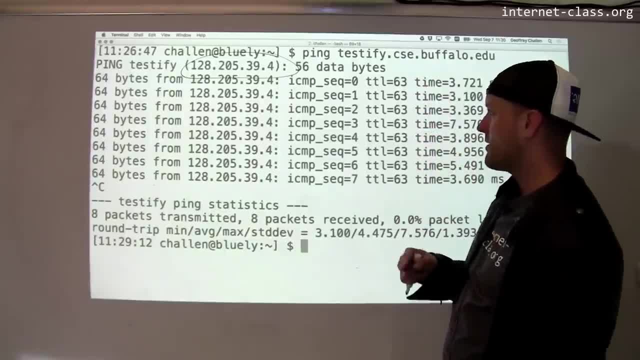 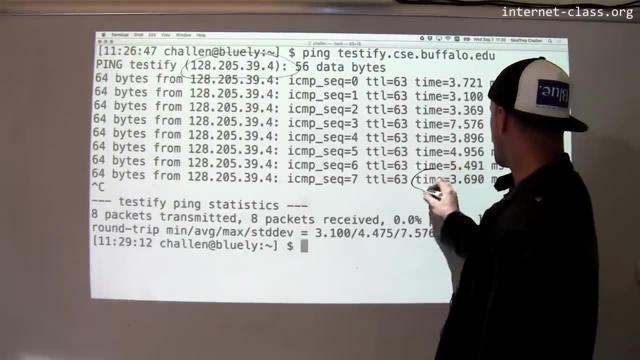 So the fact that it's 63 indicates that there's probably a very, very short connection between my computer and Testify- And hopefully there is, because Testify is in the next room, And then this gives you some information about how long this took. 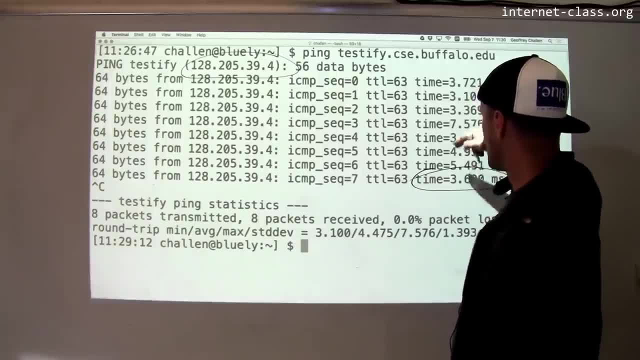 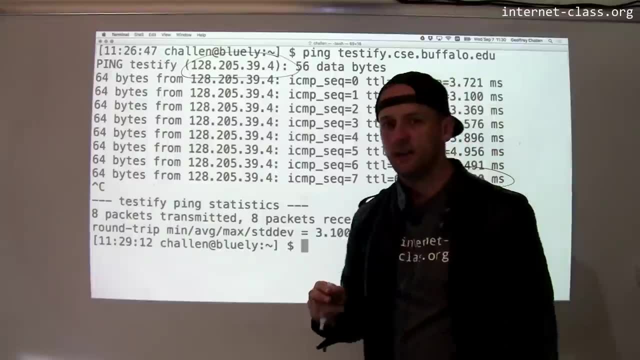 So this is about three between. It sort of varies a little bit between three and up to maybe five, or actually this one was pretty slow. seven and a half milliseconds, That's how long it took to get data from one end to the other. 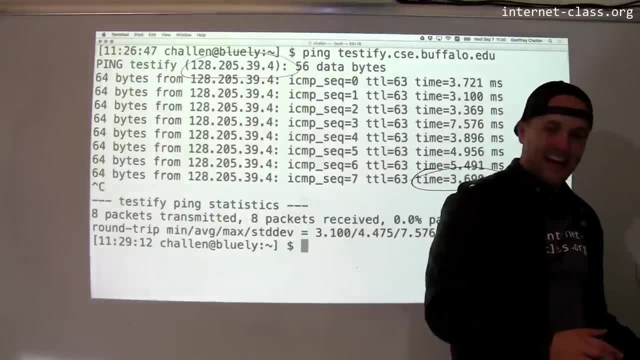 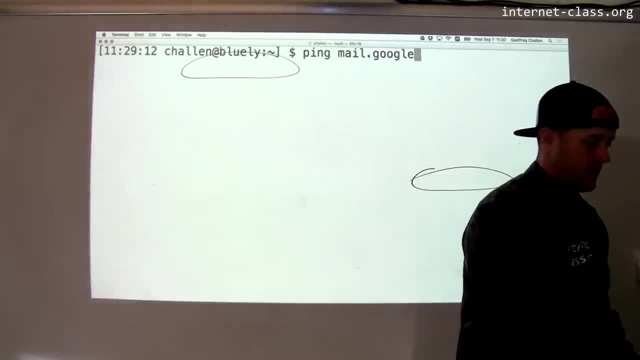 And so this is commonly used to sort of identify reachability. Not every computer on the Internet will respond to ping messages. A lot of them will. Let's try this. Let's try pinging mailgooglecom. So that's kind of interesting, right. 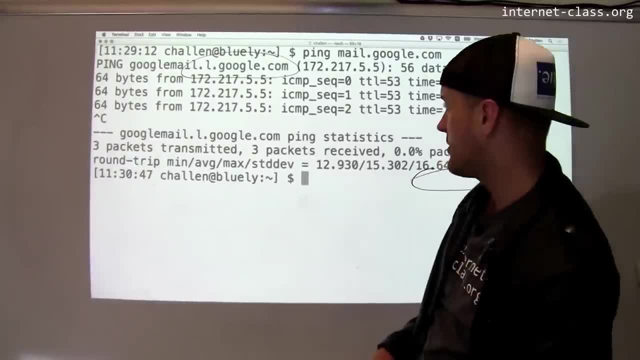 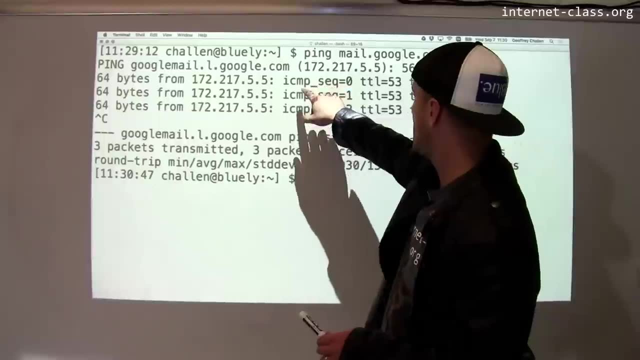 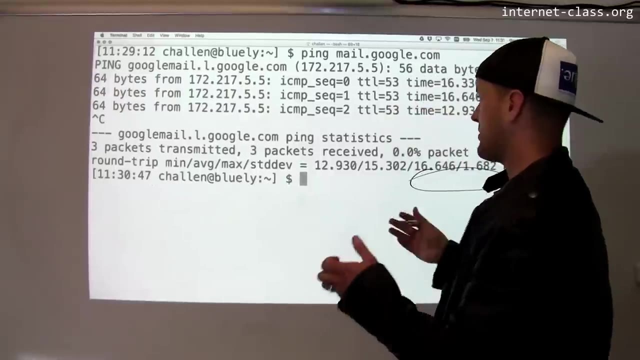 So I can actually ping, in this case one of Google's servers. So this is a machine that's hosted at Google. You can see that mailgooglecom was translated to this IP address: 172.217.55.. They probably use multiple machines to provide this particular service. 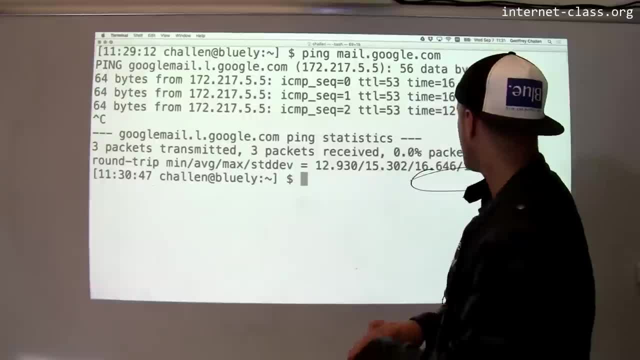 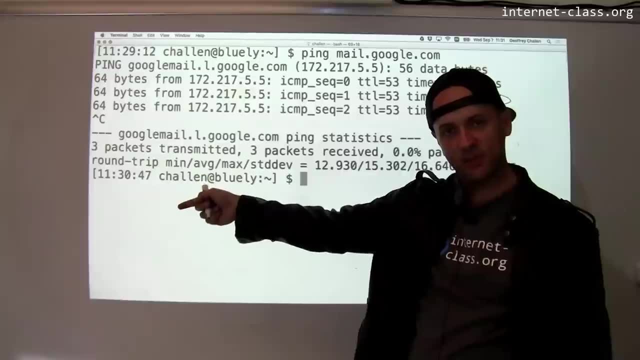 One interesting thing here to notice is that the time that it takes to ping that machine is quite a bit longer than the time it takes to ping the machine in my office. That makes sense. At some point the speed of light starts to play a role. 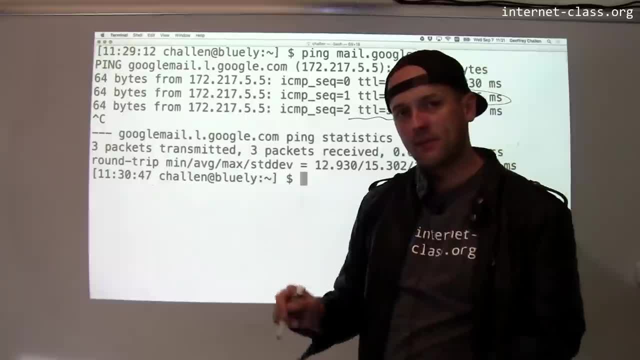 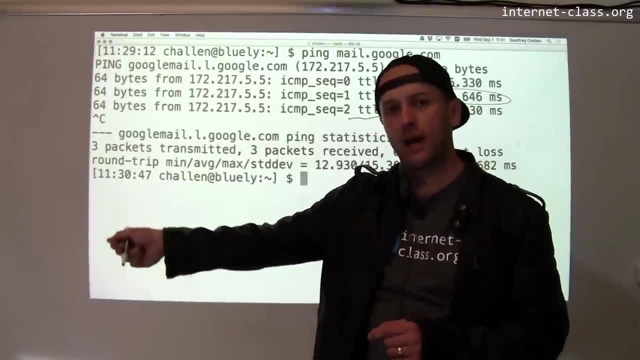 The time to live on the packet is also lower. So this indicates that this packet, rather than almost directly being sent to the computer in the next room, actually was routed by multiple routers across the Internet in order to reach this particular computer. So this is an example of ICMP.